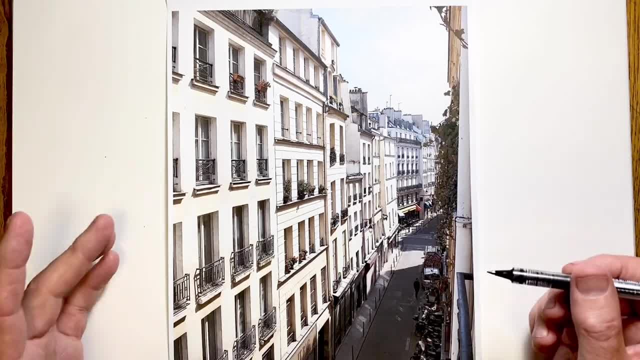 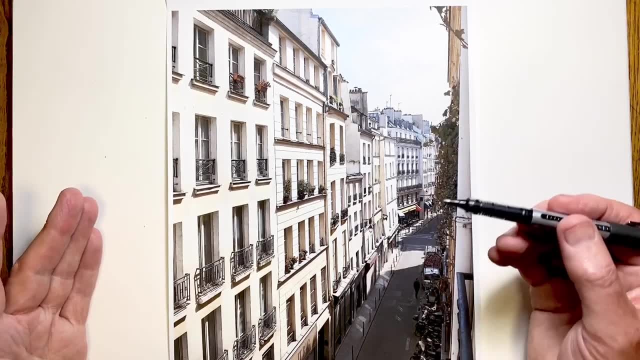 The first important thing to find in any scene is the straight ahead point. The straight ahead point is the point directly in front of the person looking at this scene, or the spot level with the camera that took the photo. It may not be in the centre because photos are often cropped. 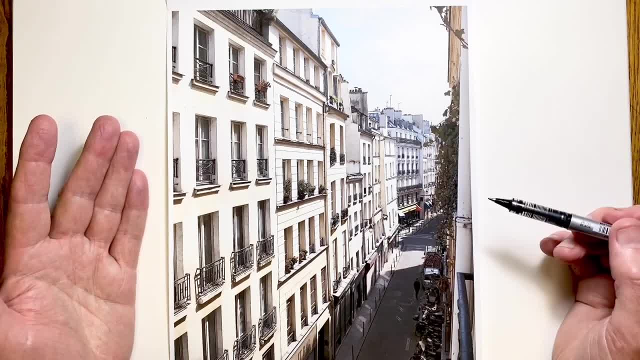 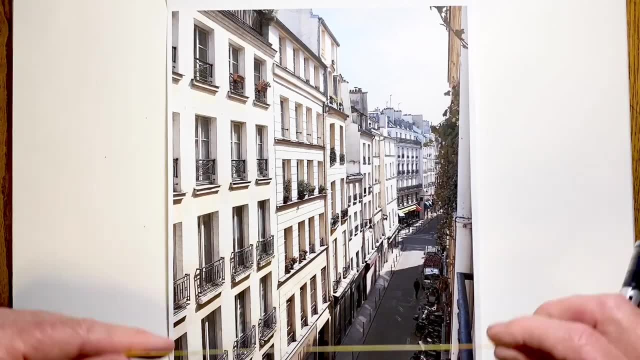 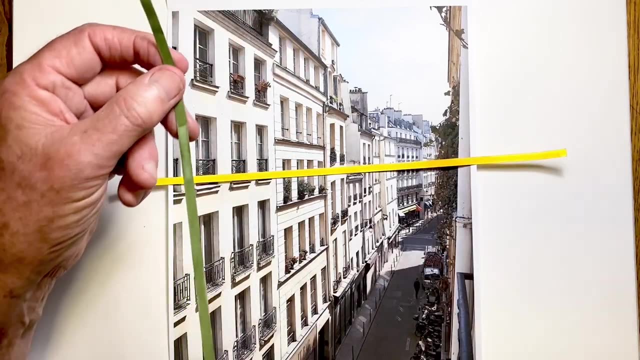 The best way to work out where the straight ahead point is is to look for where the horizontal line and the vertical line meet. So the horizontal line, the line known as eye level, is here where we have a horizontal line in all of the perspectives, And the vertical line is where we have a 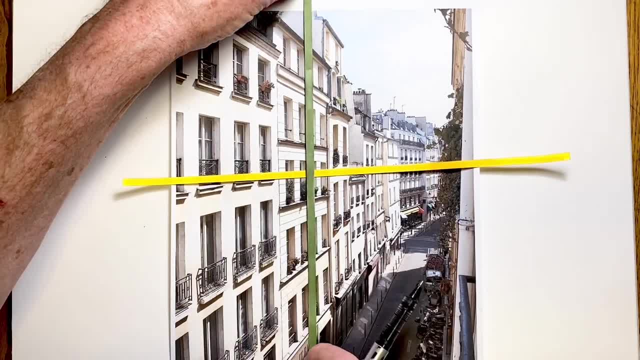 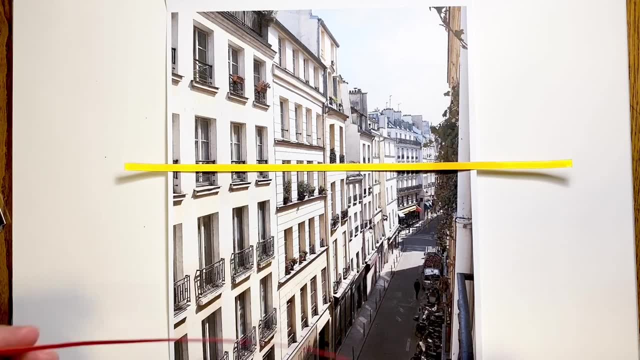 vertical line, which, in this case, is here. There's the straight ahead point. The pattern. it's not thinking about it in terms of one and two point perspective. It's thinking of it in terms of pattern. The pattern is: we look for the highest. 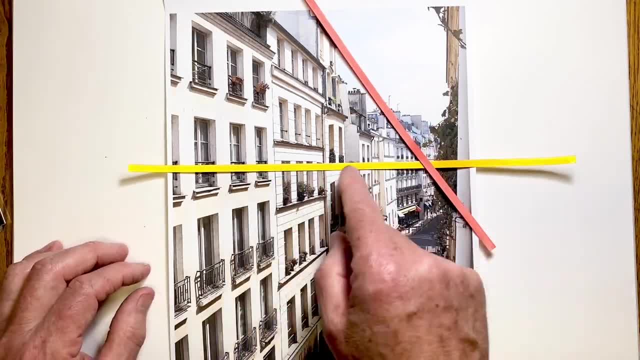 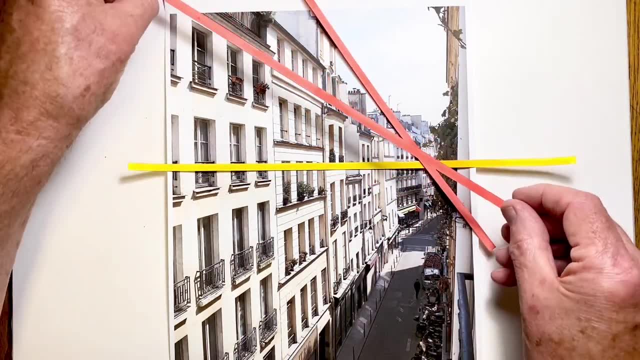 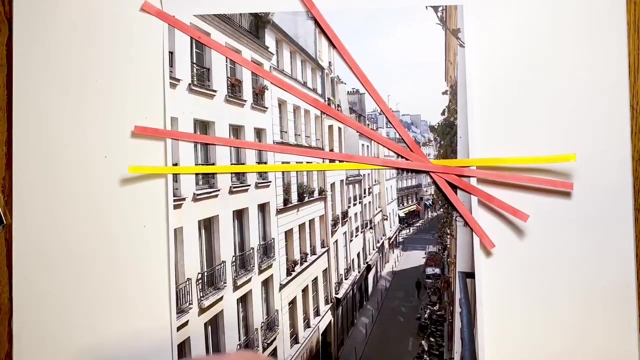 perspective line, above the viewing point, above the eye level, And then every horizontal line between this line and the horizontal line has to angle in, The angle has to decrease, And so you have this pattern of decreasing angles. And that's the pattern. we have to make sure that. 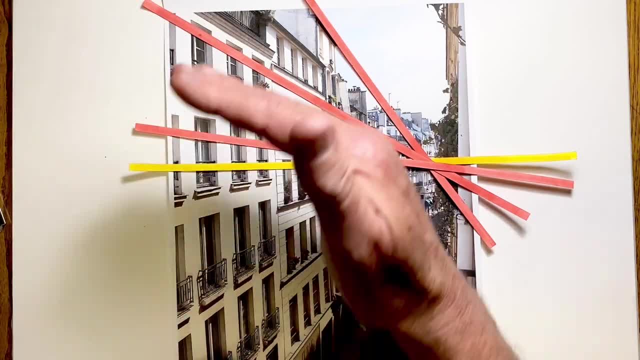 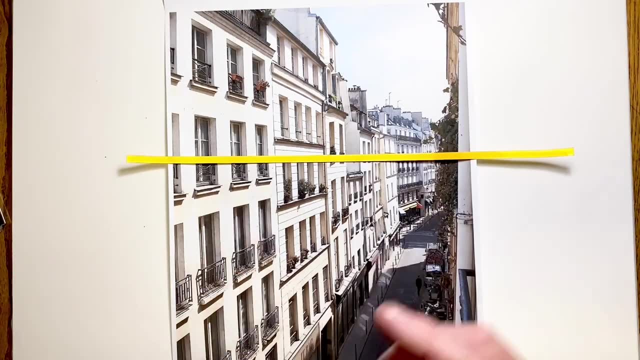 every horizontal line in our drawing follows That every horizontal line fits between the one above and the one below, But of course this pattern also works under eye level. So again, we take one of our lowest perspective lines, which is the gutter of the street, and every horizontal line. 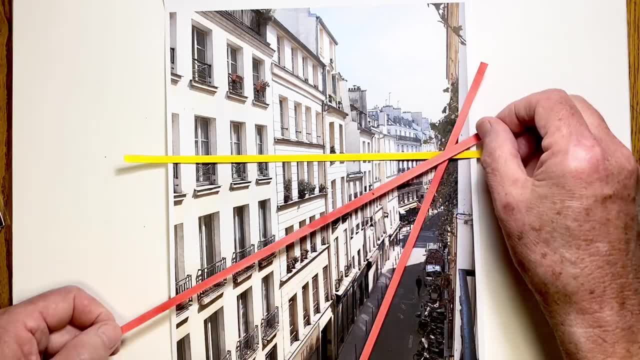 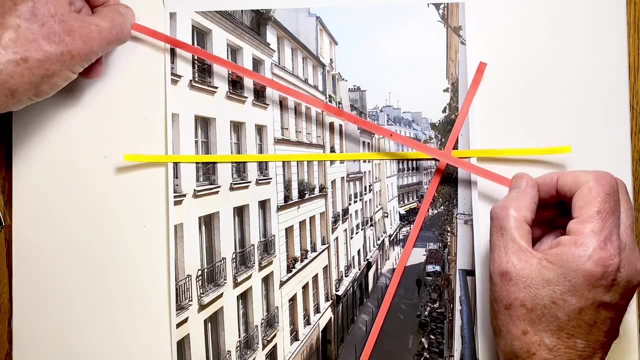 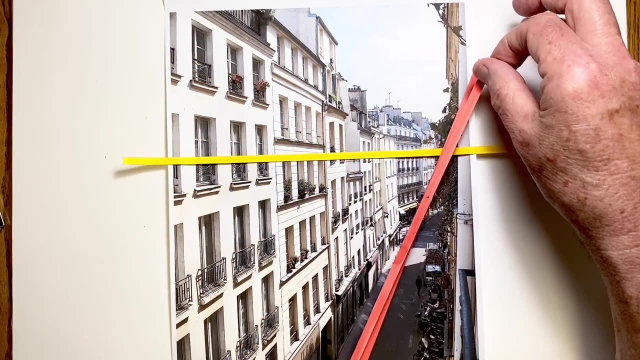 above that the pattern is that the angle increases and increases until it becomes horizontal. And then, of course, if there are still more lines, the pattern is that the angle increases, increasingly, Increases, increases, And so getting this fan of lines. so seeing all these perspective lines as 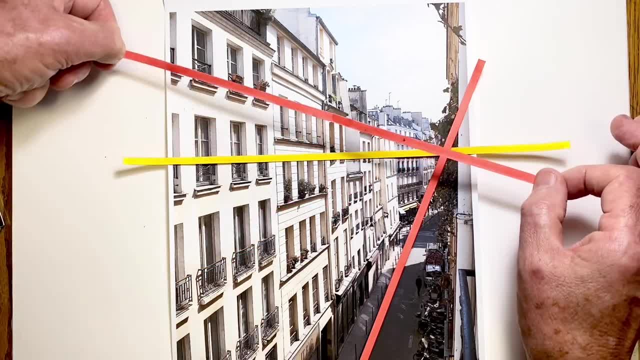 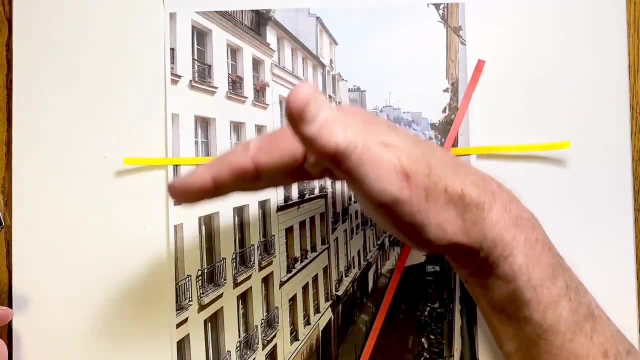 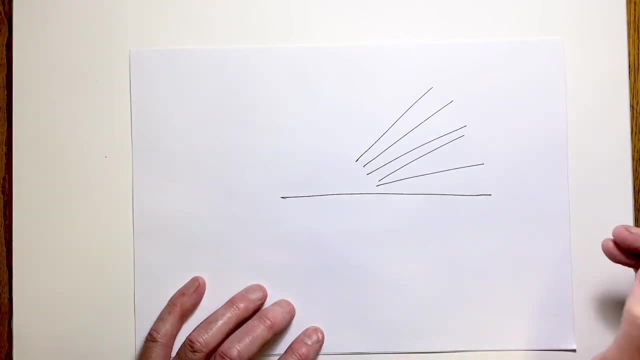 a fanning out of lines above and below the eye level line is the pattern that we need to do And if we're looking for that pattern, if there's a line that's not in the right place, it's easy to see Which line is out of place, Which line isn't in the pattern. Obviously it's this one. 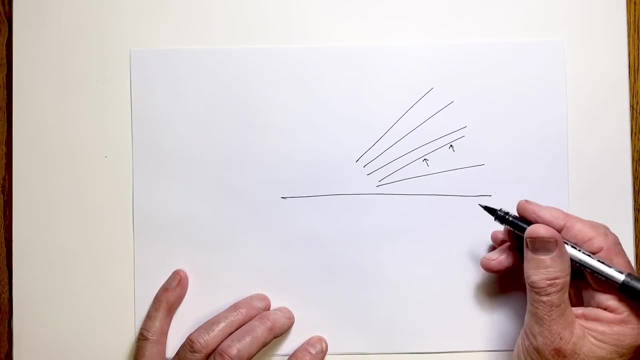 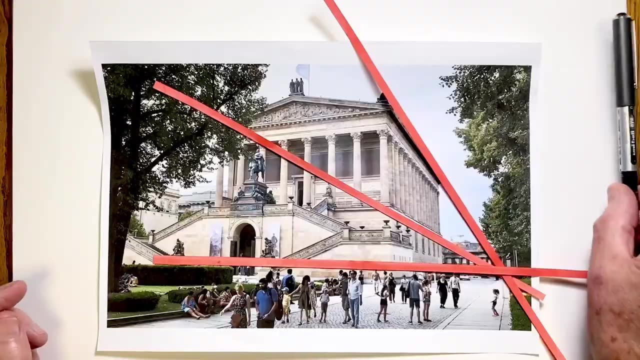 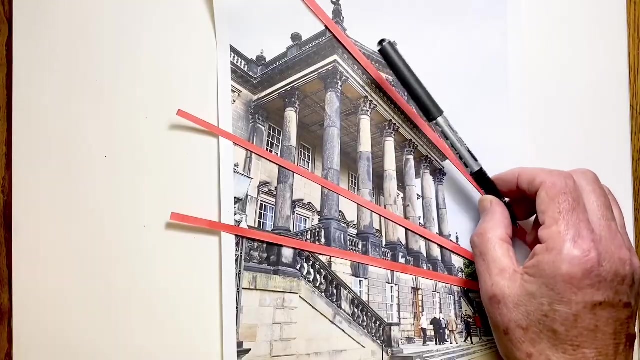 We're looking for patterns, It's much easier to see a line that isn't quite in the right pattern, And this fanning pattern can show itself in a number of ways. There may be relatively few of these lines fanning out, Or there may be many of them. They may be very steep lines Or the 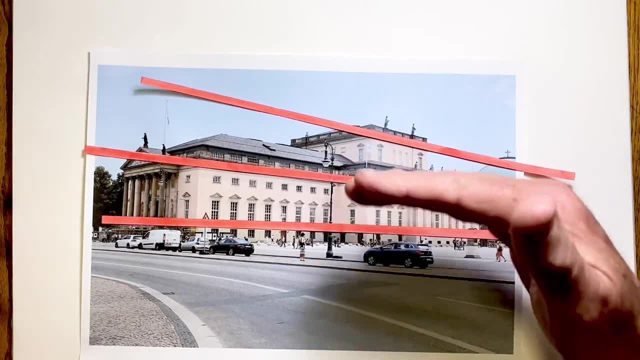 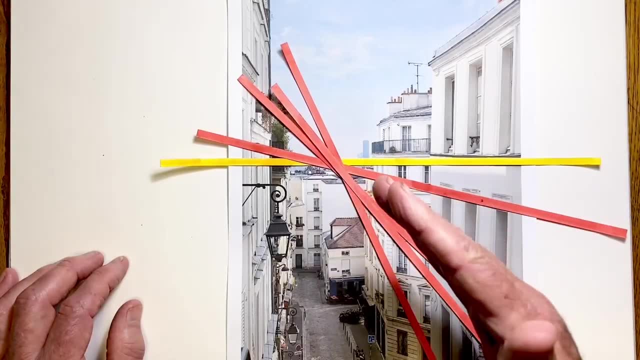 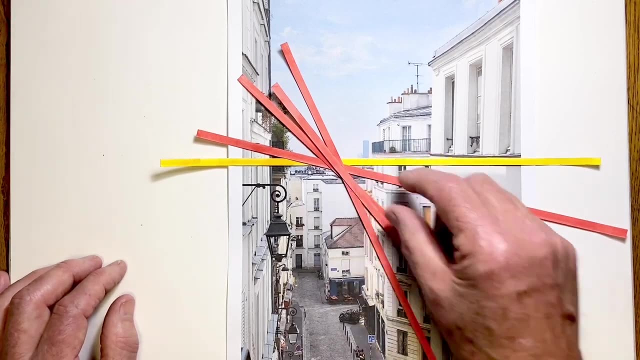 fanning out pattern of angles might be much more subtle. Most of them may be above the eye line Or most of them may be below the eye level, But the pattern is always the same. Sometimes the lines create a wider wedge and sometimes they create a thinner wedge, But the wedge shape is always there. 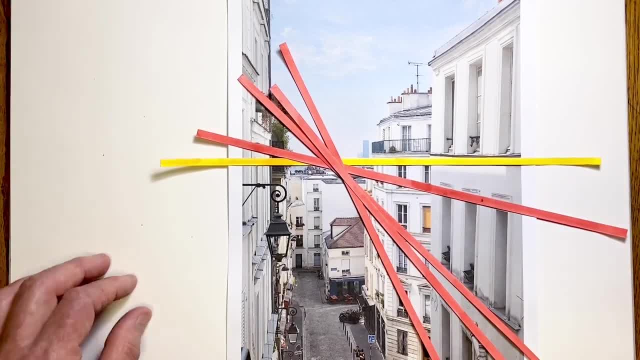 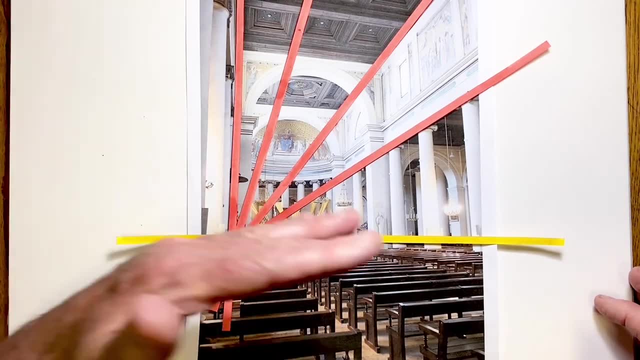 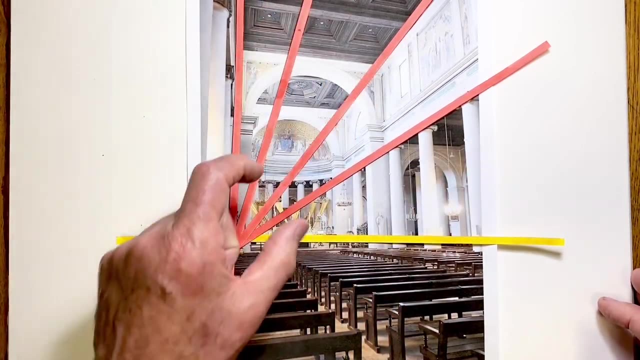 as the angles slowly increase or decrease And it's looking out for that pattern, And sometimes the perspective lines can actually roll right over the top of us, But the pattern is always there. The angle is always increasing, increasing, creating these wedges. Whether we can see the end of the wedge or not, we can see that the angle is always. 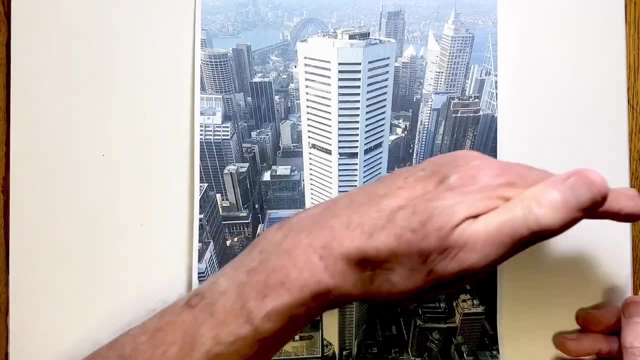 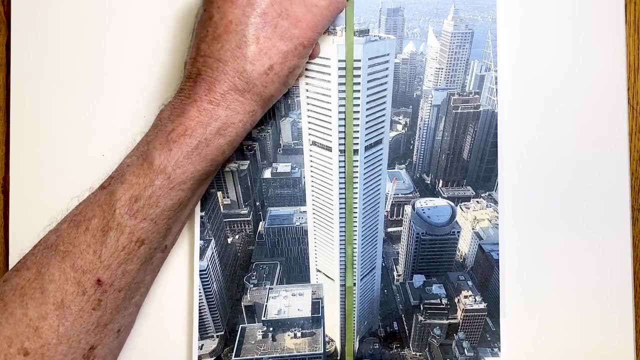 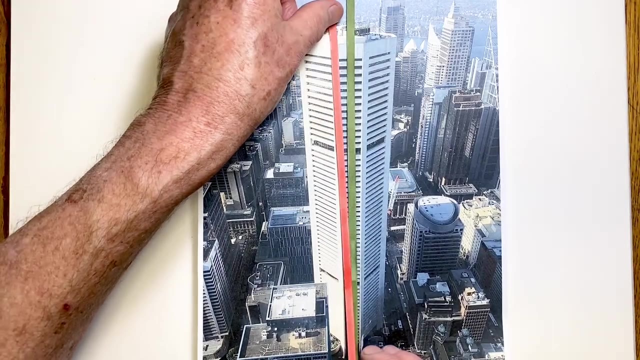 increasing. But of course a straight ahead point is not just on a horizontal axis, It's also on a vertical axis. We have a place straight ahead where, instead of being horizontal, the lines are vertical. But the pattern is the same As lines move away from the vertical, from the eye point. 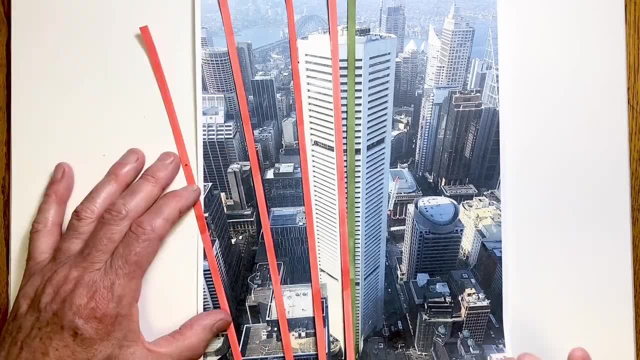 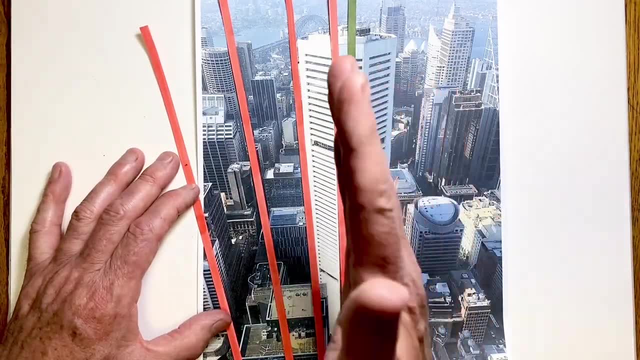 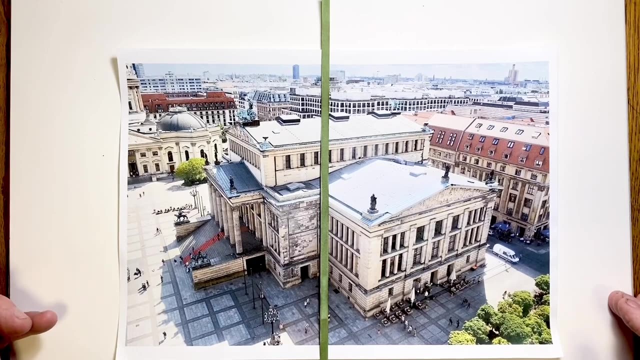 the lines are created again, simply in a different direction, And again we see the pattern that as we move away from the vertical straight ahead point, the lines increase in angle, Whether it's to the left or to the right, And it's not just in tall office blocks that we see the straight ahead point. 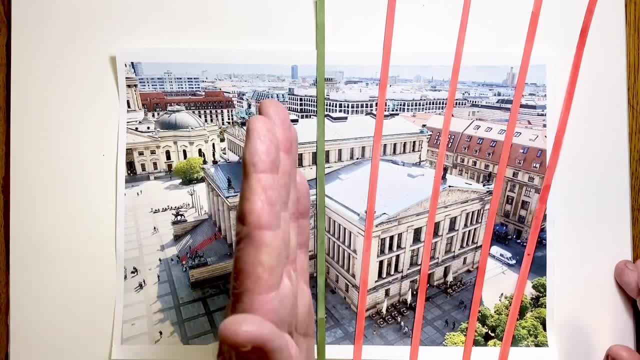 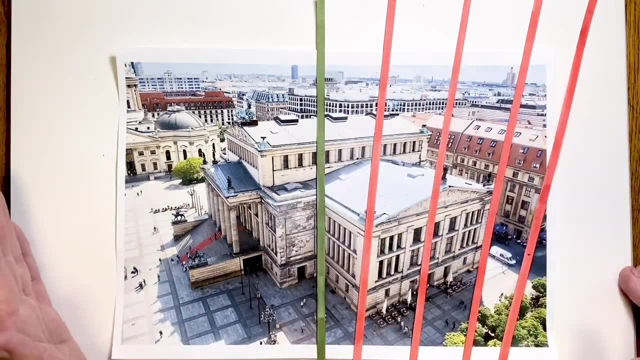 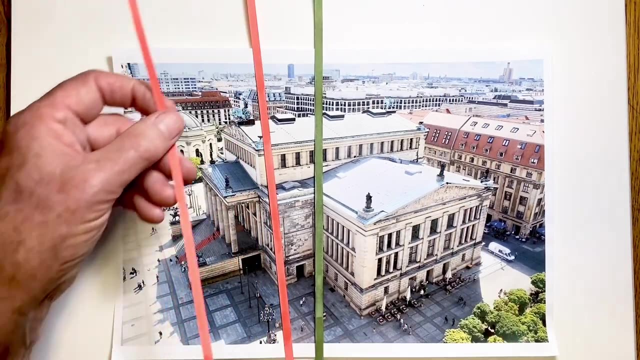 And again we can see that vertical lines to the right of the straight ahead vertical axis slowly increase in angle as they move away away from that straight ahead vertical axis And, as you've doubtless guessed by now, if we go on the left-hand side, 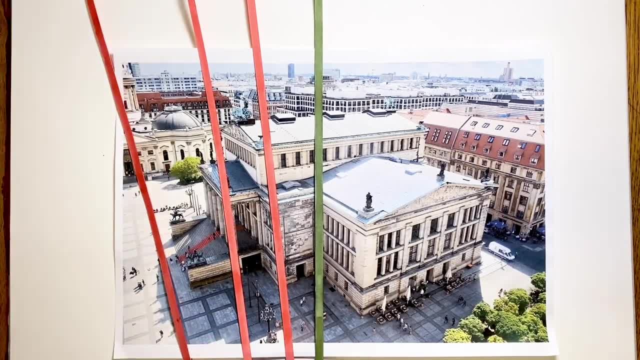 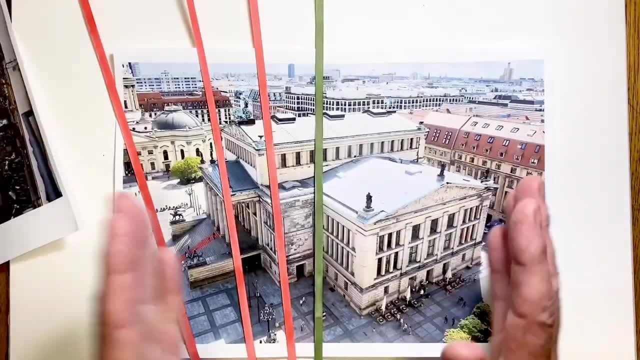 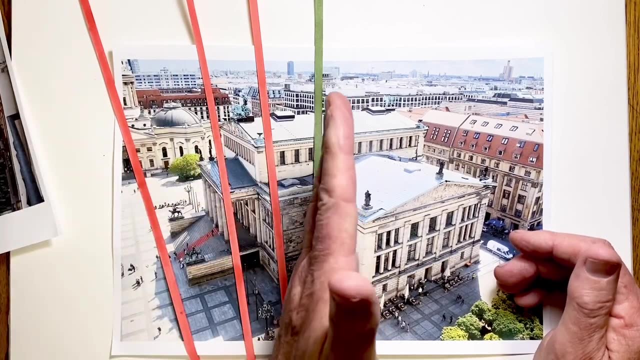 of the straight ahead vertical axis, we have the same effect happening. So this is the pattern, whether it's on the horizontal or whether it's on the vertical. It's that same pattern of increasing angles as you move away from the vertical or the horizontal straight ahead axis. 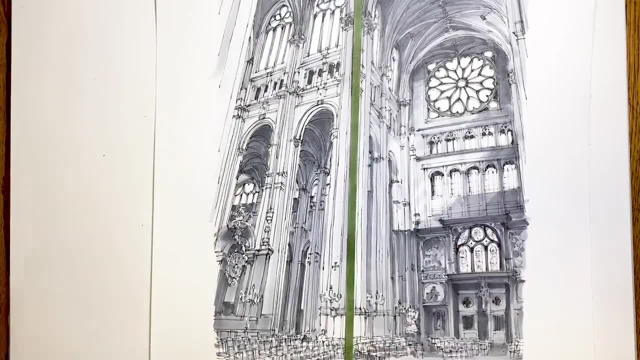 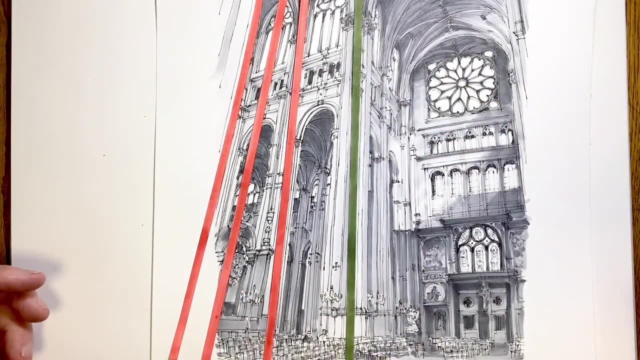 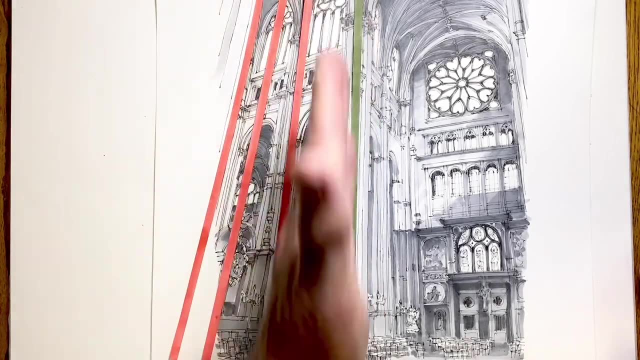 And it works with the vertical straight ahead axis in the opposite direction, when the lines are converging upwards rather than downwards in our previous vertical examples. And again the same pattern on the left-hand side as the lines move away from the vertical straight ahead axis. 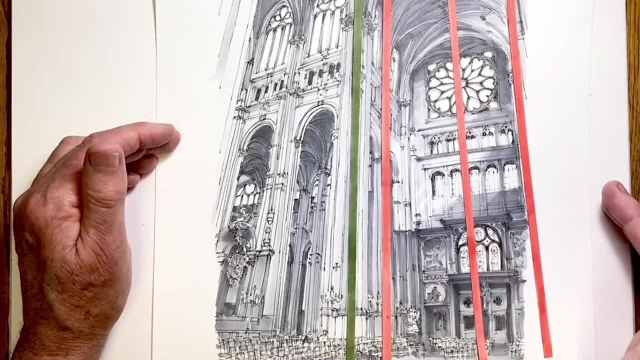 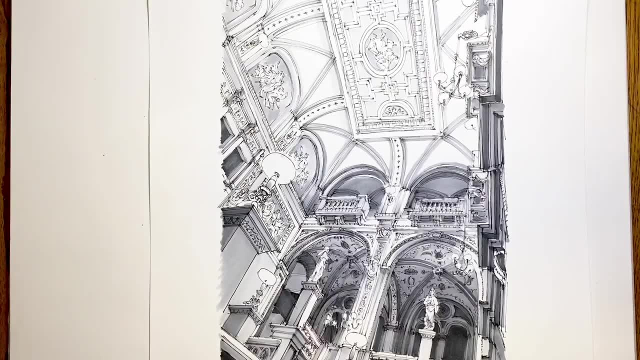 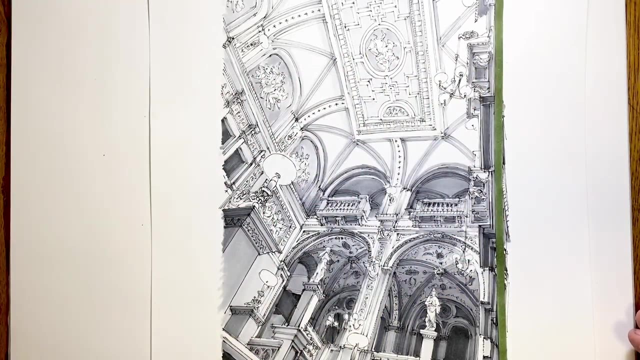 And it's the same pattern of slowly increasing angle on the left-hand side. In this case the angle is slight, so the wedges end up being much longer, And sometimes the vertical straight ahead axis can be right on one side of our field of vision. 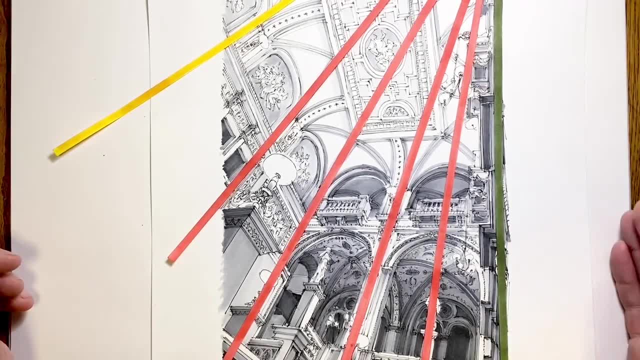 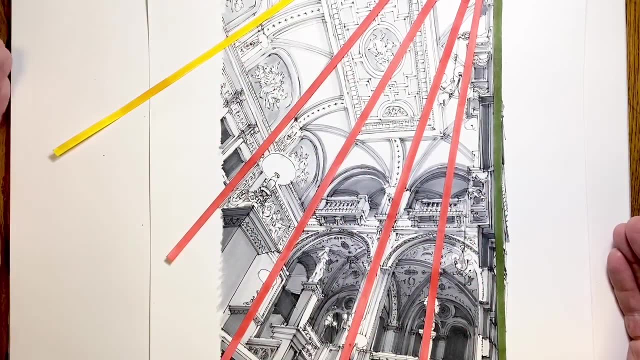 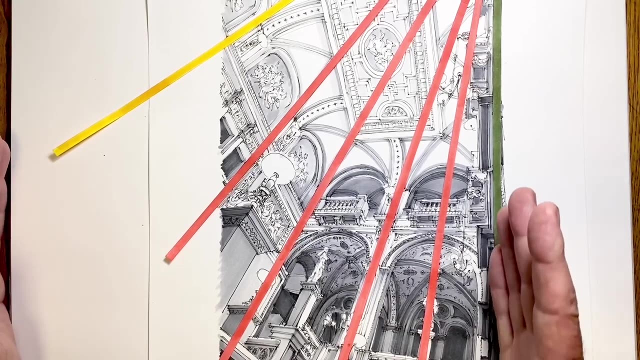 And so the true vertical may be right on one side and all the angles increase in one direction only across the entire vertical plane. What that means is, when I took this photo looking up in the Vienna Opera House, I was actually standing right hard against the wall, looking upwards. 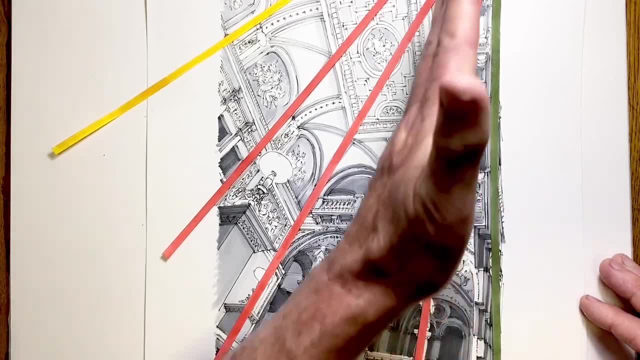 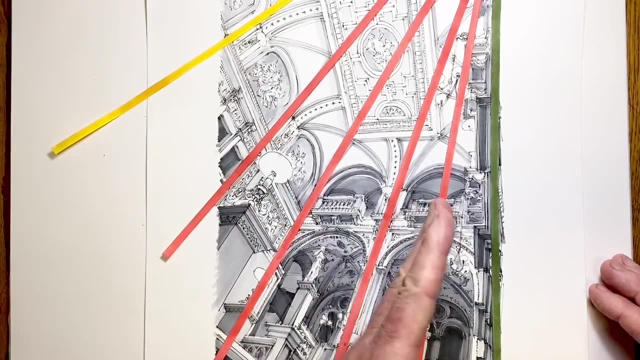 But again, when I draw this, I see the pattern, So that every vertical line has to be increasing in angle from the one before it. And that's the pattern. I'm looking for both in my reference, whether it's real life or a photo. 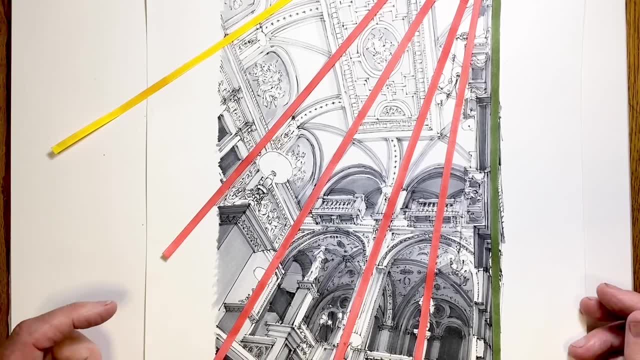 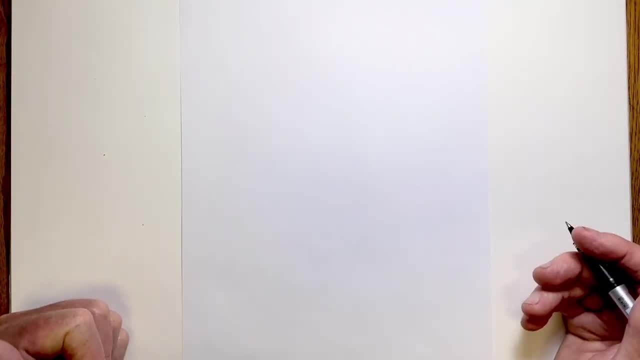 and my cross check to see if I've done it correctly is to say, is there a line that doesn't fit into the pattern that stands out And there are other perspective patterns to look out for? Here's a column that's made of various segments. 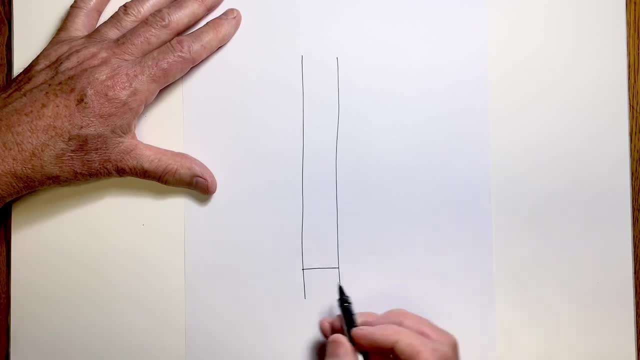 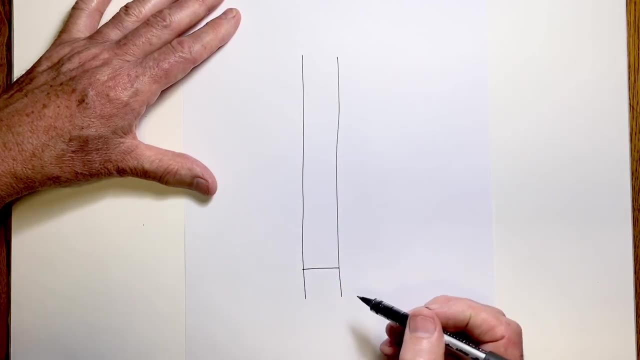 And here is our straight ahead viewing point. So we have a horizontal line there. Now, if this column is made up of various cylindrical sections stacked on top of each other, then we know this is actually a circular line in real life, Although straight ahead it looks flat. 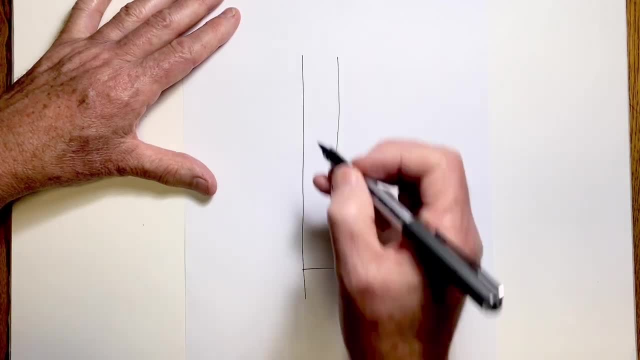 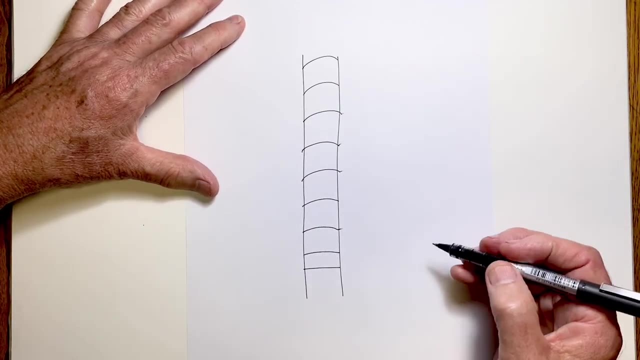 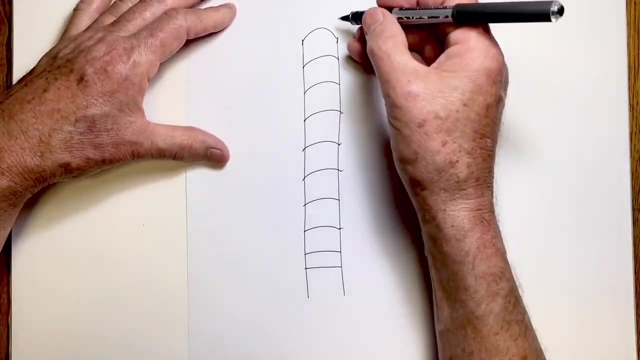 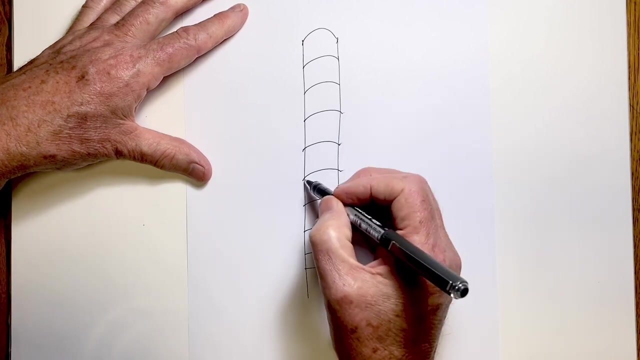 But as circular lines move up above the straight ahead point, the pattern. the pattern is that the line becomes more and more rounded the higher it goes, And so that's the pattern. And so again, when I'm doing my drawing, I can make sure I'm thinking I must increase the curve. 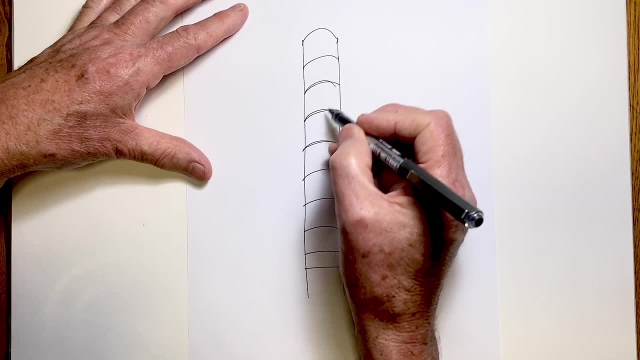 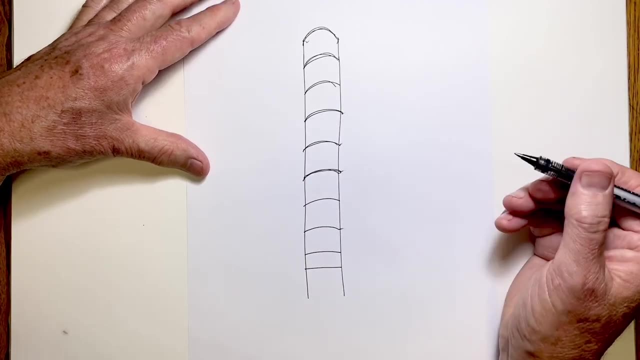 with each of these lines, even if it's just a little bit. And I find thinking that way in terms of the pattern of the increasing curves is a very good way to keep me accurate in drawing. And if we look at a real life example, 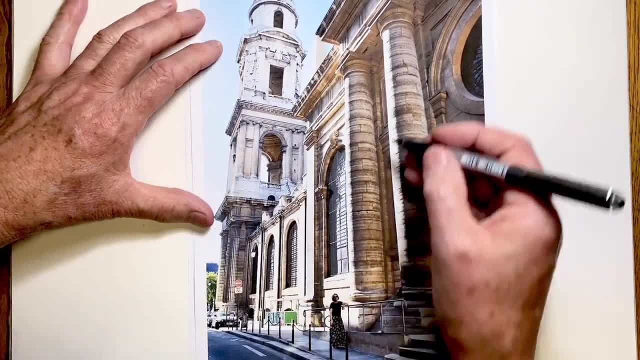 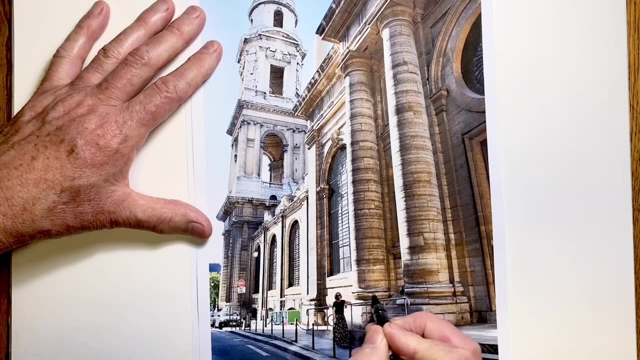 we can see that this is in fact the case. Here's one of the massive side entrance pillars. It's at St Sulpice in Paris And we can see here the straight ahead line that's actually on the base of the column. 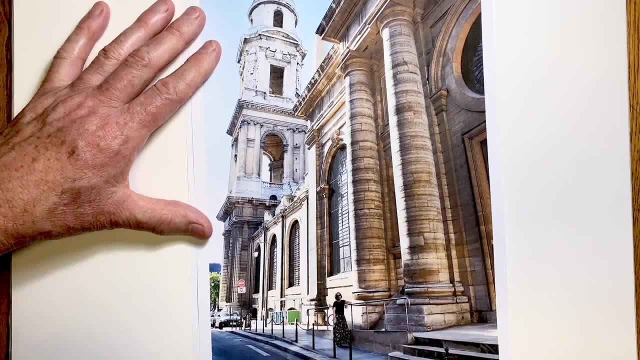 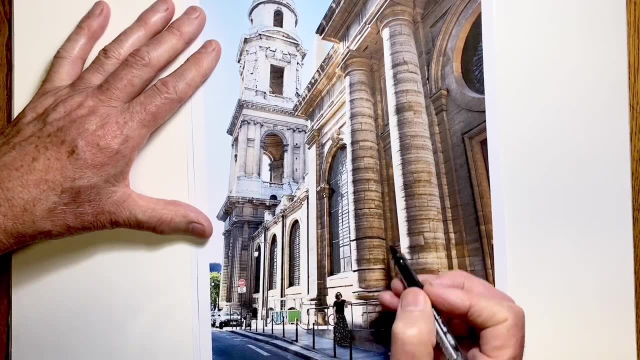 And it lines up with the eye level of this person here And we can see that there's just a very slight curve there. If we go a bit further up, it's a bit more. If we go a bit further up, it's a bit more. 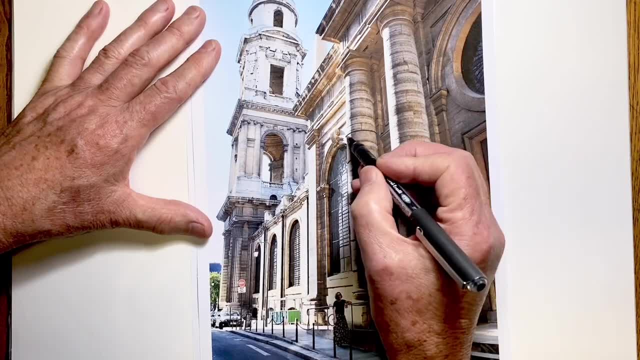 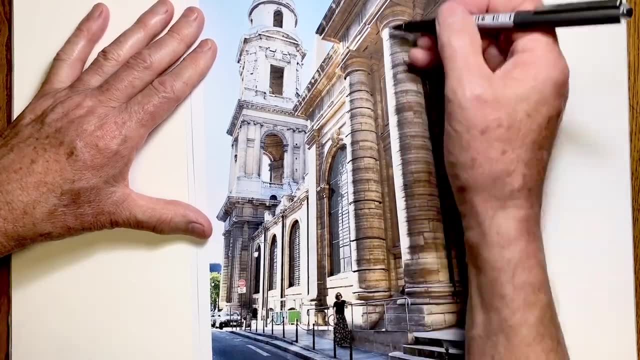 If we go a bit further up, it's a bit more, And we can see that this pattern, in fact, is what happens in life. And, of course, it's not just in columns that we need to be thinking of this pattern If we have a building, such as the dome of a church. 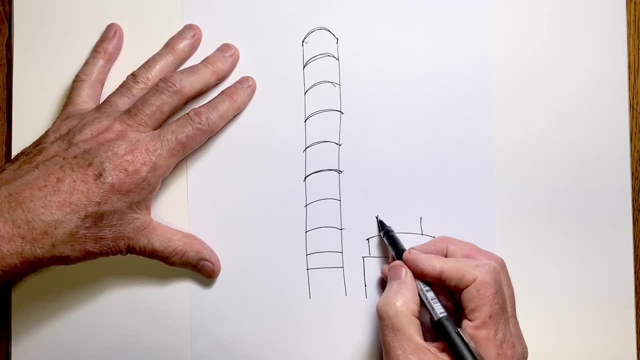 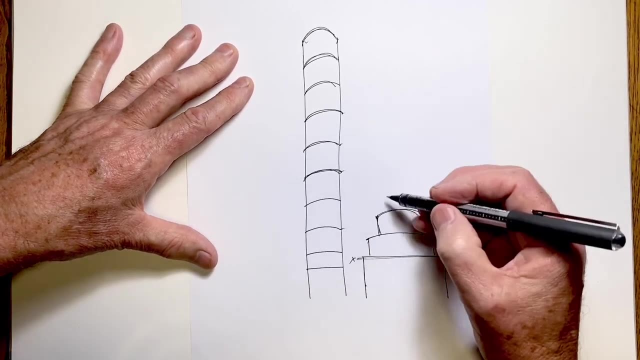 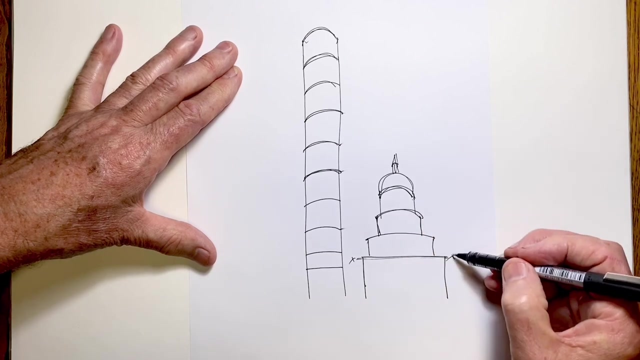 and it sits on a number of drums. as the drums get higher and higher, they're moving further away from our eye level And therefore the line increases. And again the pattern is as these circular lines move further away from our eye level. 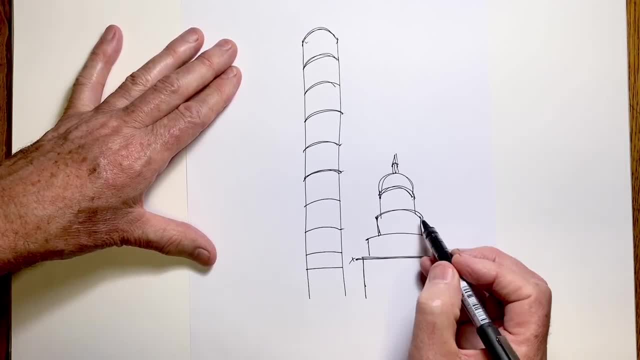 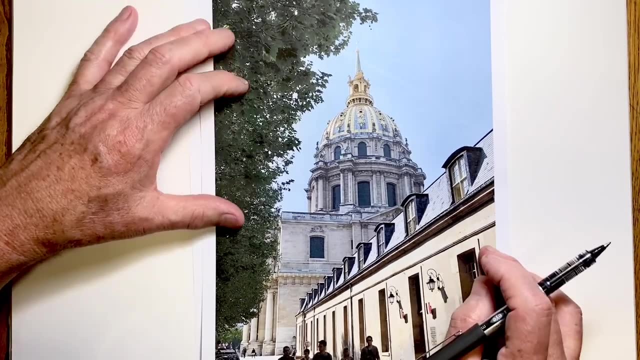 And again, the pattern is: as these circular lines move further away from our eye level and further away from the straight ahead eye point, the curving gets more and more pronounced. If we look at life, we can see that this pattern is there. 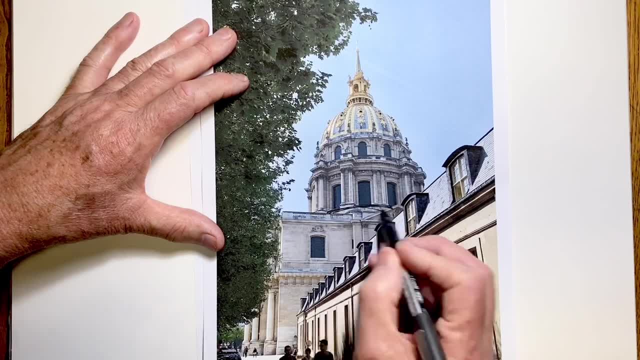 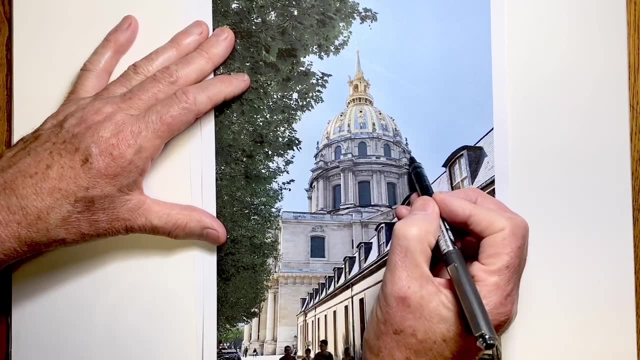 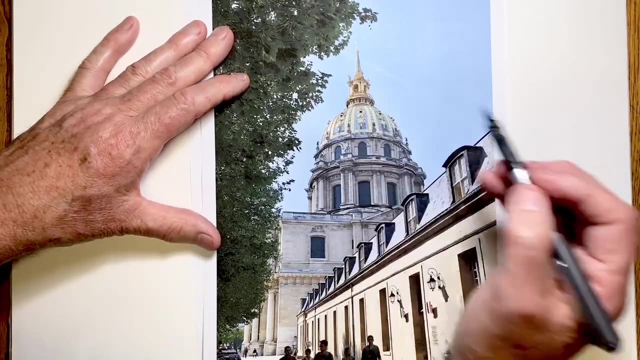 We can see that this line here has less of a curve than this line here. We can see that this line above it has more of a curve And we can see that this circular line here, although it's a much smaller circle, has a much more pronounced curve. 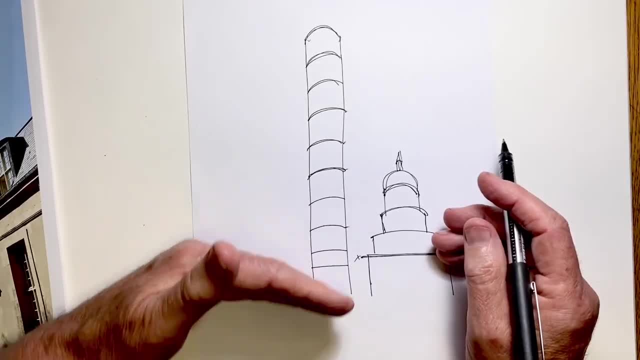 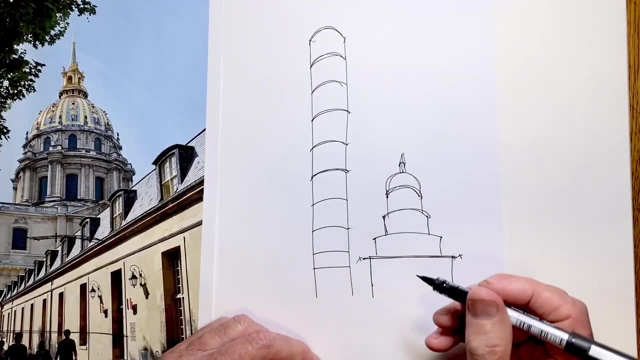 So we can see. in fact, this is how this works. If we remember that this is the pattern we need to look for when we're observing our reference photo and when we're drawing, we can make sure we have added attention to making sure that we increase these lines as we go up. 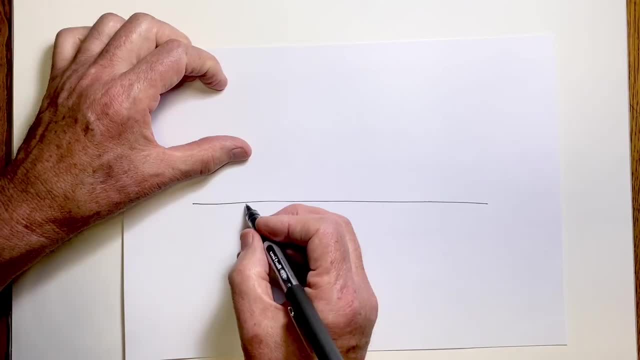 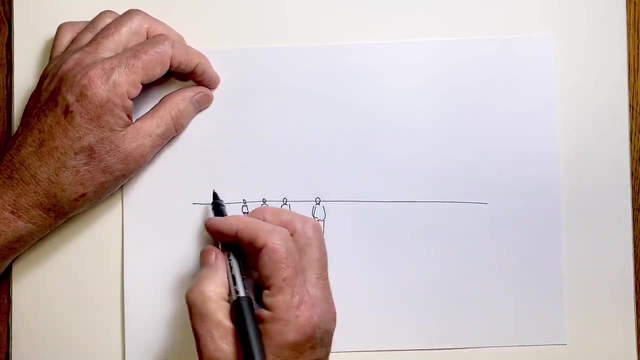 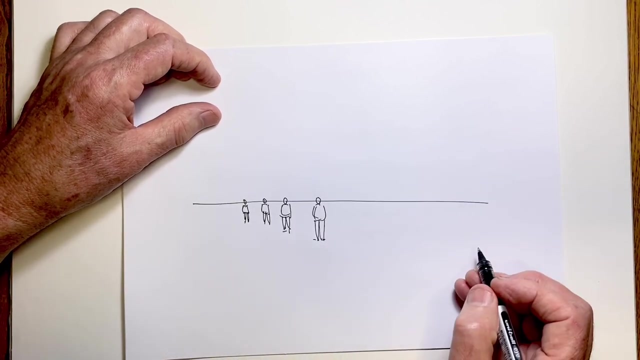 There's a very important pattern with people as well. When we're looking at a crowd of people, the heads all line up in a straight row, As long as they're all approximately the same height and as long as the ground they're on is flat. 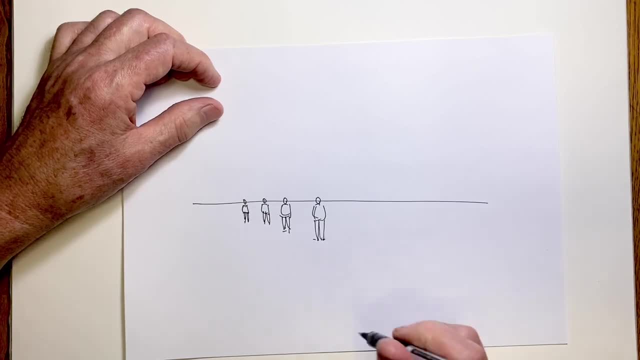 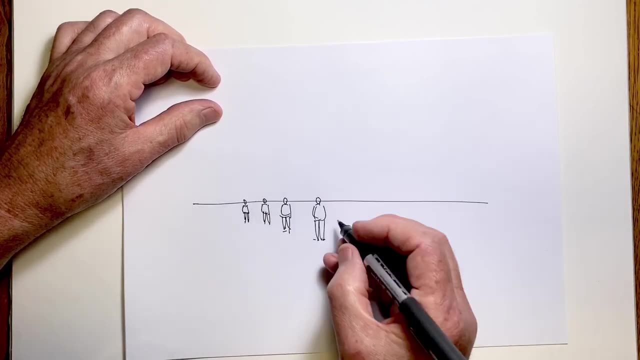 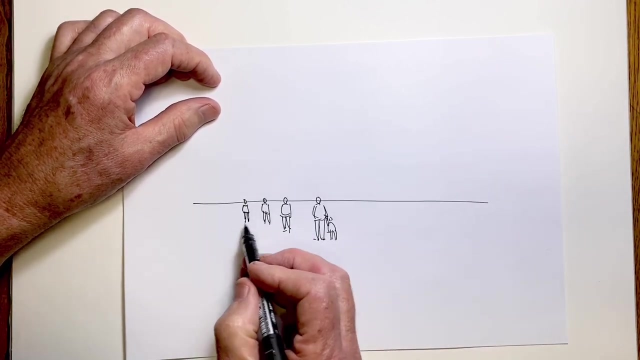 and I'm looking at them from the same flat ground, So my straight ahead point lines up with their eyes, which puts all their heads in a straight line. That doesn't work if there's a child, because they're not as tall, And so the pattern is the heads are all on a straight line. 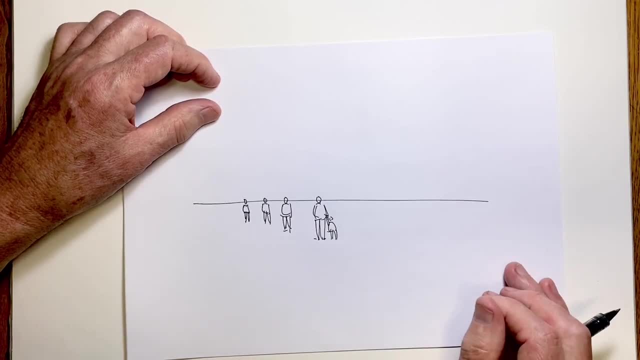 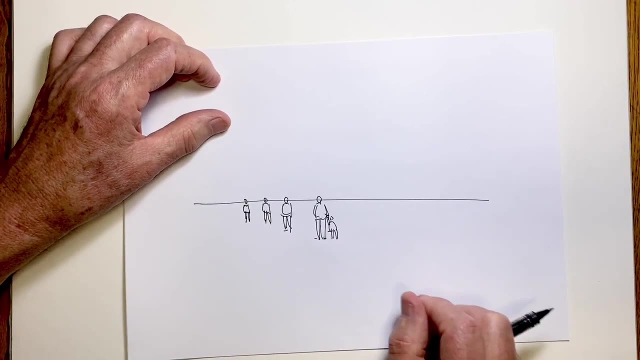 and the feet are at different levels. And again, if I remember this pattern when I'm looking at my reference photo or my life scene, it helps me to see, it helps me to pay attention to what's really there, which is the fact that the heads line up. 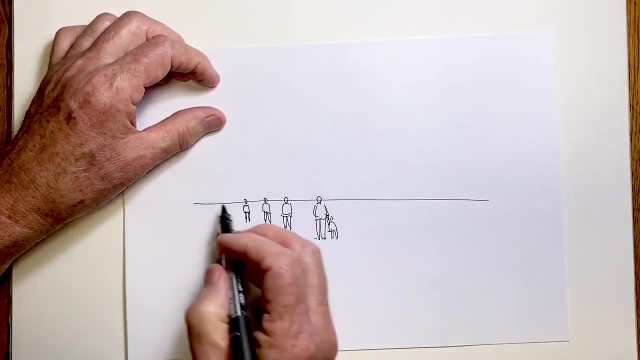 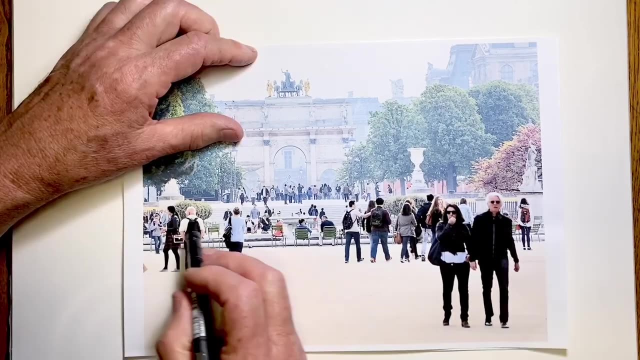 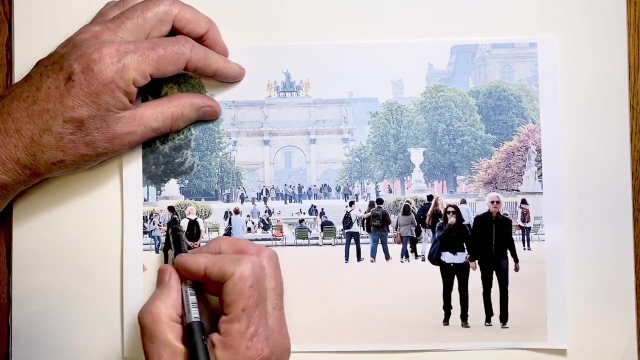 the feet have to become further and further away from the straight ahead point, the closer the person comes to me. Look at that in real life and we can see all these people in this front section who are all on flat ground- the same level. I was on when I took this photo. 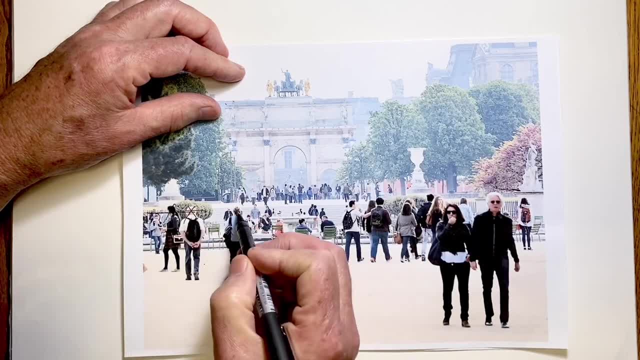 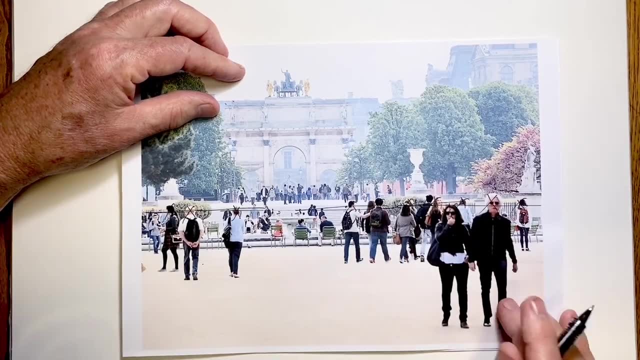 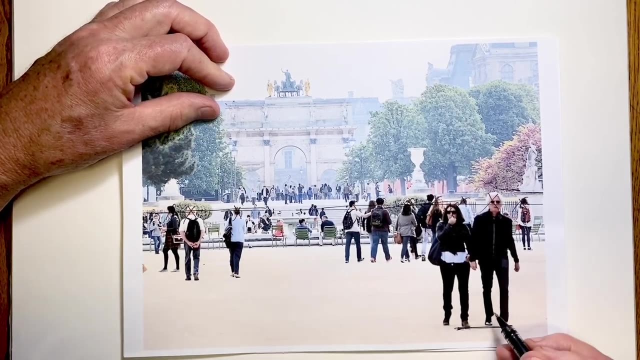 We can see that their heads, their heads, pretty much all line up, even though they're at quite different locations, And we can see that the feet of the people closest to us are the lowest and the feet of the people furthest away from us. 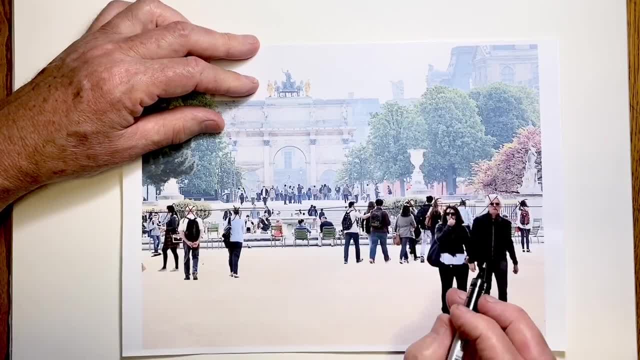 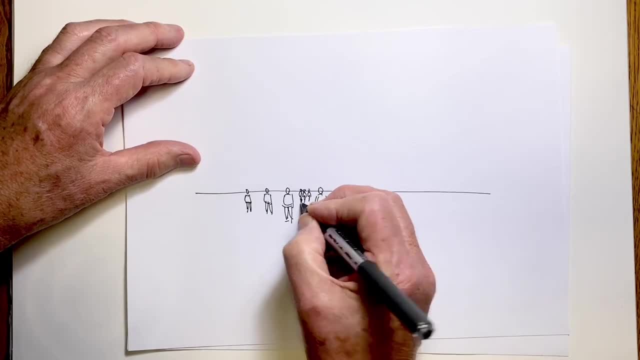 are the highest up. But by thinking in terms of this pattern, when we're observing the crowd we're going to draw, it's easier to see it accurately, And then when I'm drawing, I'm aware of keeping all the heads on the same. 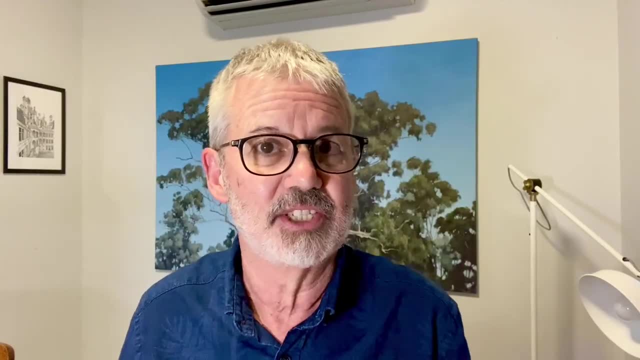 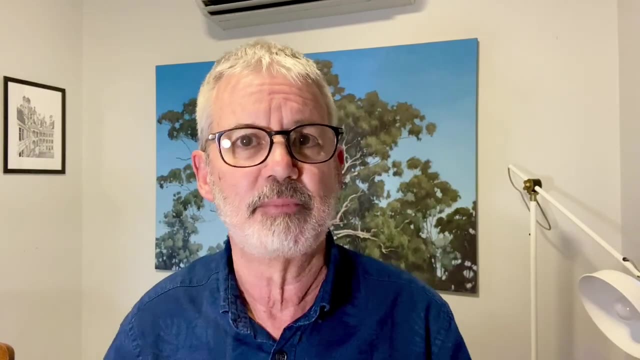 straight ahead level. Well, this is how I do it. When I draw, I don't think about those perspective diagrams and vanishing points. I look to see the perspective patterns that have been formed from the viewing position with that particular subject And I use those patterns to help me see. 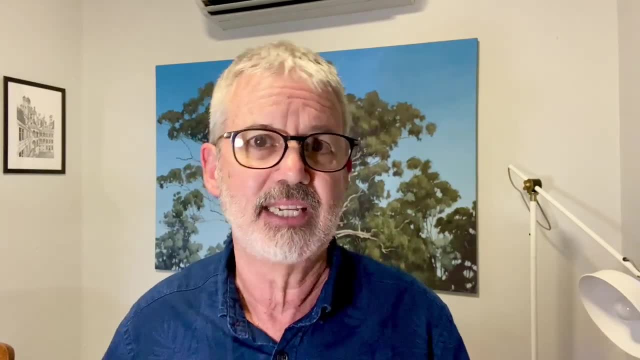 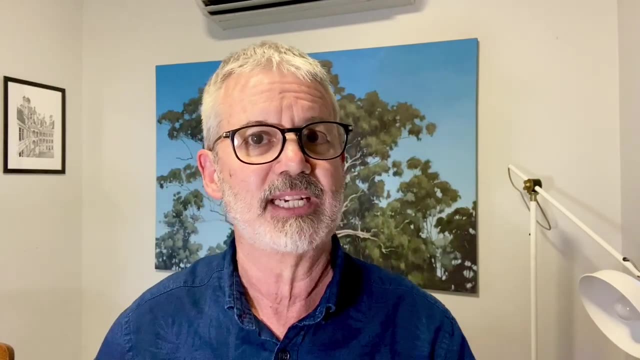 what's happening more clearly Now. these were some of the simpler patterns in this video. In my next video on perspective patterns, I'll be looking at some of the slightly more complicated patterns that perspective throws up, And maybe this just adds to the confusion for you. 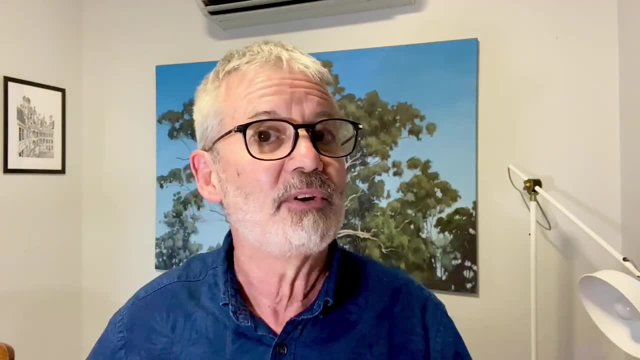 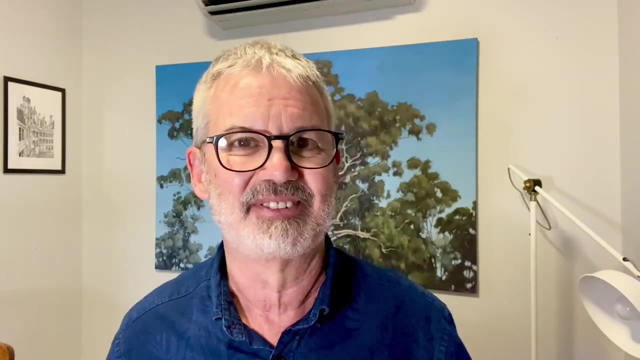 But for some of you, I hope it gives you a new way, perhaps a clearer way, to not just understand perspective but also to be able to capture it more accurately in your drawings. So keep drawing, have fun. I'll see you next time. Bye.